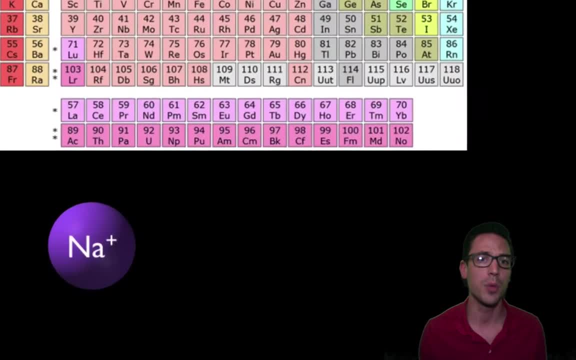 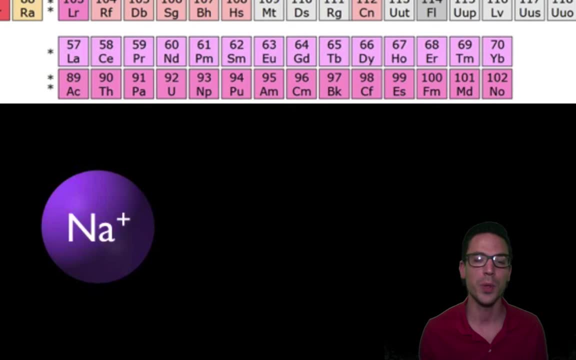 with already are sodium and chloride. So sodium, which is Na because it's on that left side of the periodic table, it has a tendency to lose an electron. it typically is gonna have that positive or negative charge, so we call this guy a sodium ion Chlorine. on the other hand, Cl has a tendency to gain an. 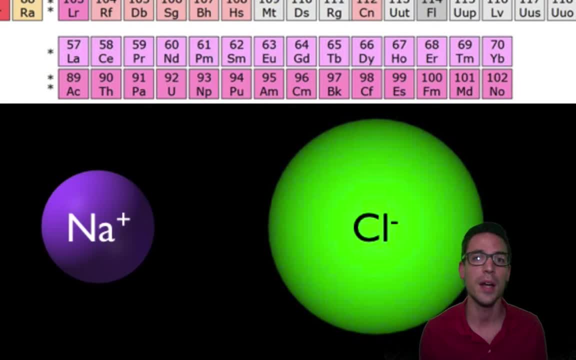 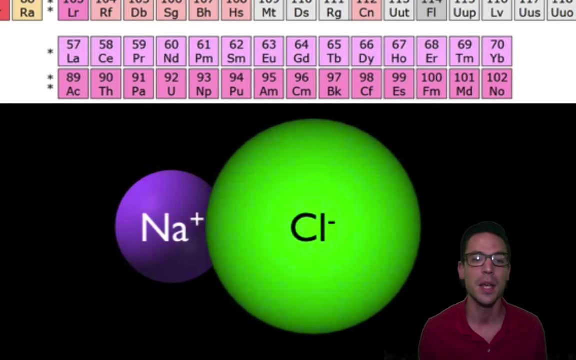 electron. so that's gonna give it that negative charge. so we'd call this guy a chloride ion. Now, if you bring a positive and negative charge close enough together, what do they do? Well, they attract and they're gonna form what's called an ionic bond. and any time that they bond together, they're 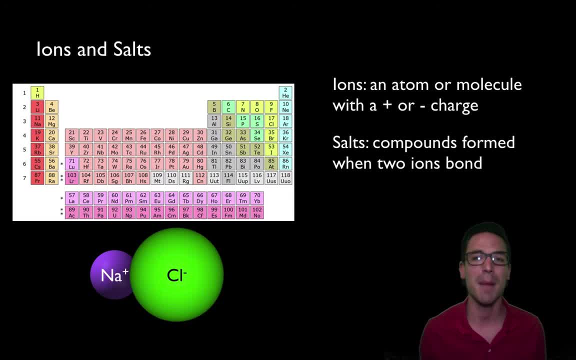 gonna form what's known as a salt. So all that a salt is is any compound formed when two ions bond together because of that positive and negative charge. So here we have sodium chloride, a salt that you're probably very familiar with. Now, if we were to look at the composition of sodium and chloride, 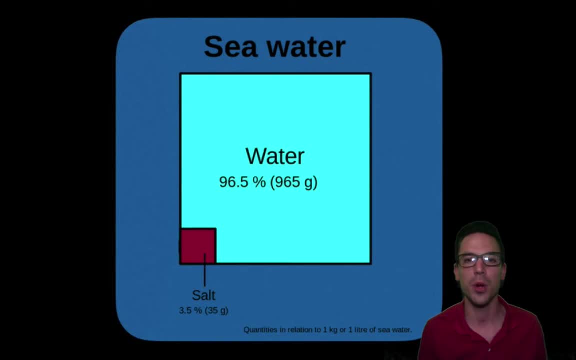 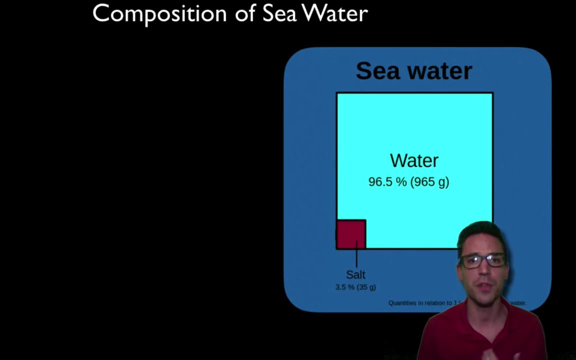 we'd notice that about 96.5% of seawater is just water or H2O. The other 3.5% are gonna be various types of salts or ions. So what sorts of salts are we talking about? If we were to just zoom in here? 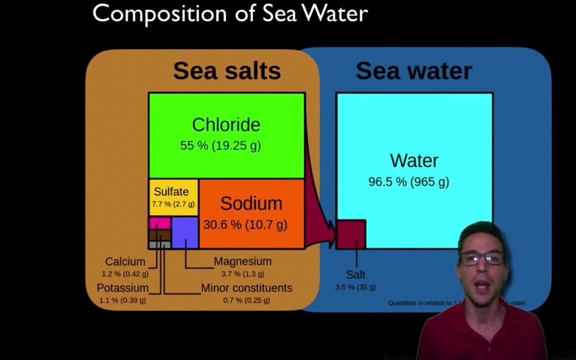 we notice that most of it is what we just talked about, sodium chloride. That's why, if you ever get seawater in your mouth, it tastes very salty. most of it is sodium chloride, But the other types of salts or ions can be sulfate, calcium, potassium, magnesium. all these things are gonna make up what? 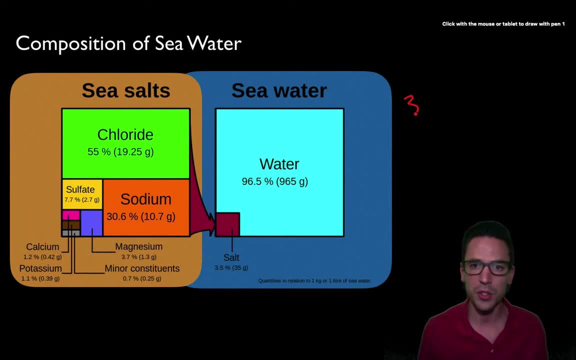 is about 35 grams of salt. These salts are gonna be found in about 1,000 grams of seawater. We say that the salinity of seawater is typically about 35 parts per thousand, or we can abbreviate that using the symbol that you see here. So typically seawater is gonna be 35 parts per thousand, but 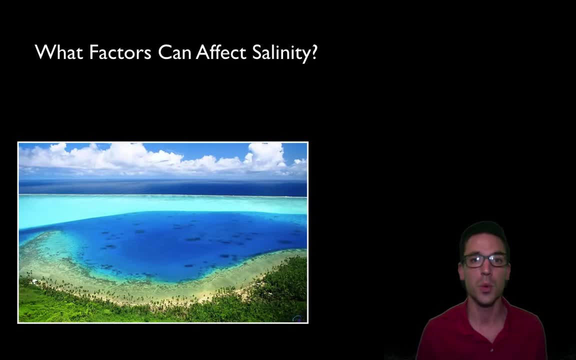 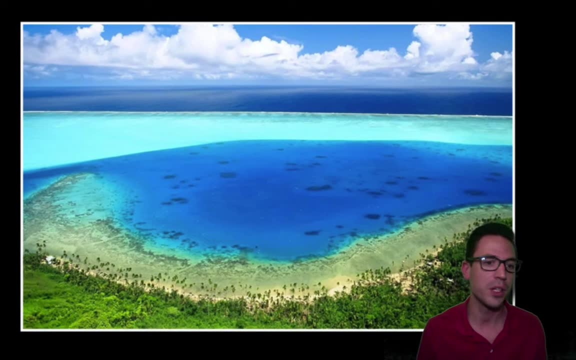 different factors can either increase that number or decrease it. So what sorts of factors can affect salinity? Well, one of them is gonna be evaporation. So here in this picture, we have a lagoon, and all that a lagoon is is a body of salt. It's a body of salt that's gonna be used to evaporate water. So 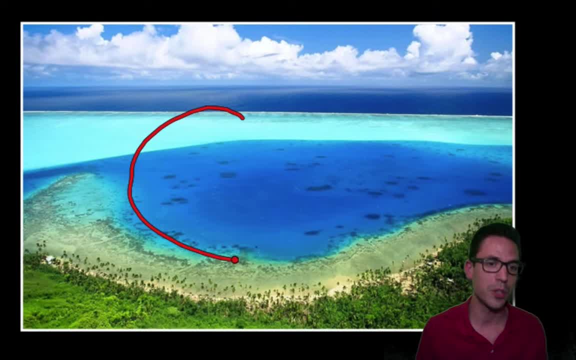 it's a body of water that is cut off from the rest of the ocean. So here's our lagoon. You notice in the background here we might have a coral reef. let's say that's separating it, so water can't come in and out. So as that water in the lagoon heats up, that water is gonna evaporate, but it's. 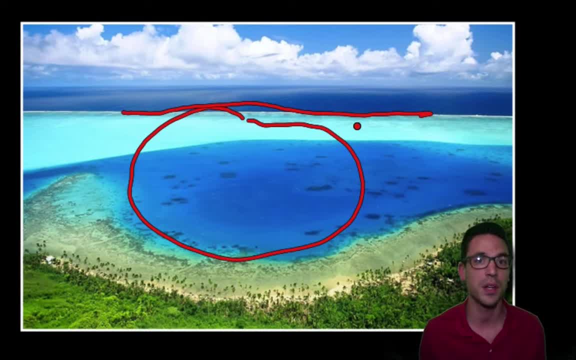 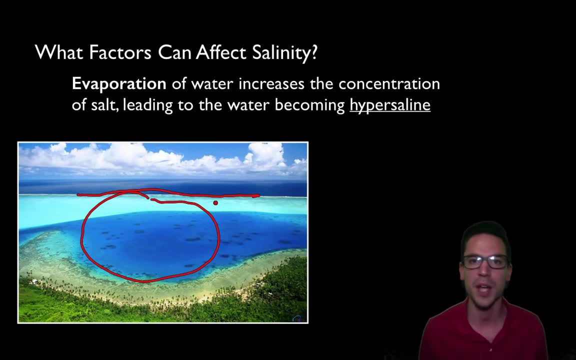 gonna leave the salts behind. So how does that affect the salinity? The salinity is gonna increase, So evaporation of water increases the concentration of salt, leading to water that we can call hypersaline. The prefix hyper just meaning above, So it's above the typical salinity of 35 parts. 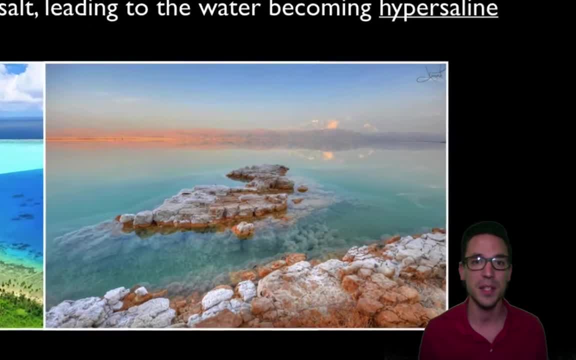 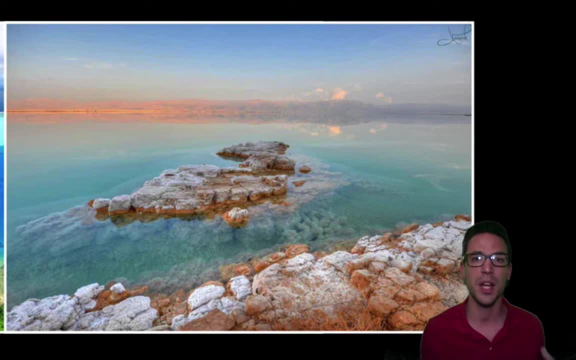 per thousand. A great example of this that we see here is the salinity of salt. This is the salinity of salt. The Dead Sea is the Dead Sea. The Dead Sea is a body of water found near Palestine and Jerusalem, And this is an area where water feeds in from rivers, bringing dissolved salts into it, but then 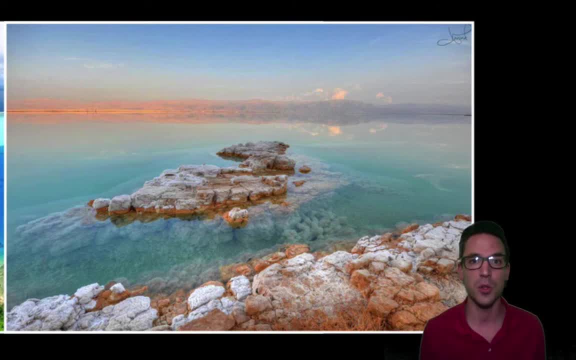 that water gets stuck there until it evaporates and then it leaves those salts behind. So over time, tons of salt has been dropped off in the Dead Sea. The water evaporates and that means that the salinity goes higher and higher. In fact, there's about 10 times more salt in the Dead Sea. 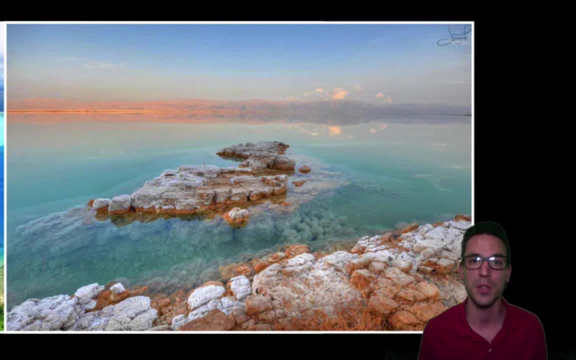 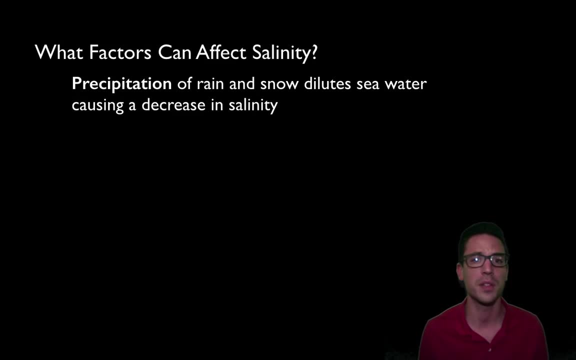 than there is in the ocean, So about 350 parts per thousand as opposed to 35. That's why it's called the Dead Sea. You typically don't find life living there. Now, another thing that can affect salinity is going to be precipitation. Precipitation is going to have the reverse effect, As it rains or snows. 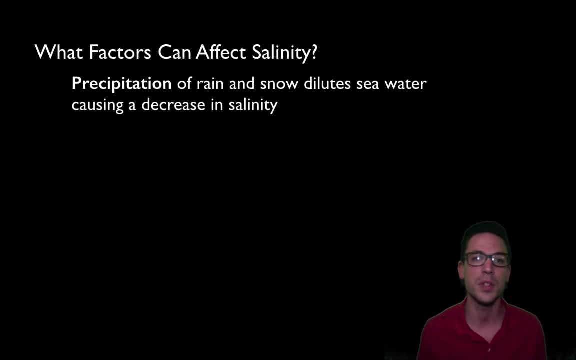 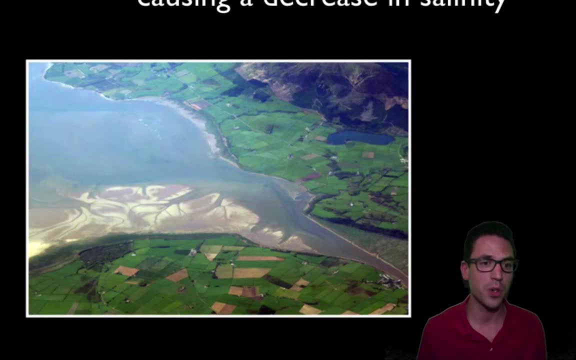 that's going to bring fresh water and that's going to dilute some of the salt and decrease salinity. This is a similar effect that we see in estuaries. So in this estuary, this is going to be where, let's say, fresh water systems, rivers, streams, lakes lead out to the ocean, So that's going to decrease. 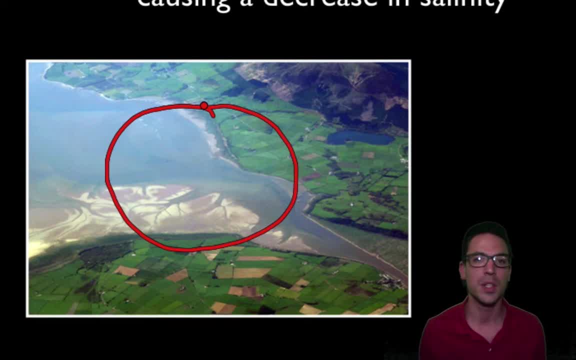 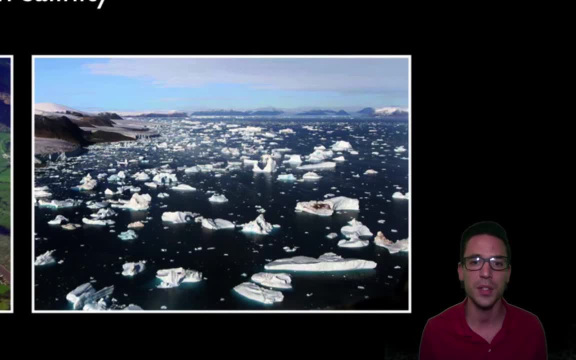 the salinity of the water. We end up what's called brackish water here, because it's not salt water. It's kind of a mixture in between. We also find that we can change salinity in areas near the Arctic where we might have a lot of ice melting. As that ice melts, it's going to dump a lot of. 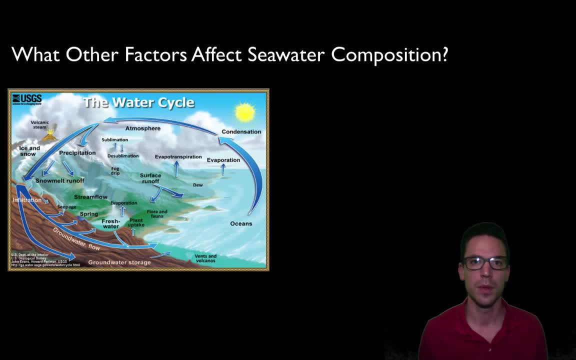 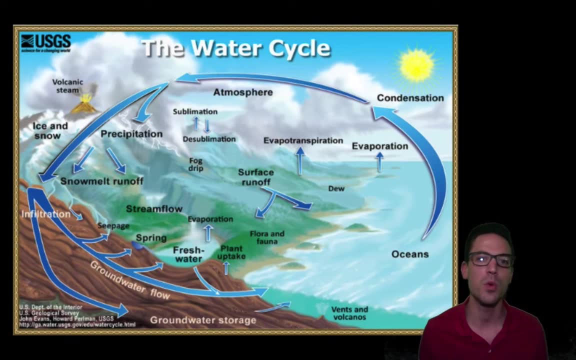 fresh water into the ocean and that's going to decrease the salinity. Now, salts are not going to be the only thing that we find inside ocean water. So if you are familiar with the water cycle, you know that water is always moving from the oceans up into the atmosphere, down into nearby rivers. 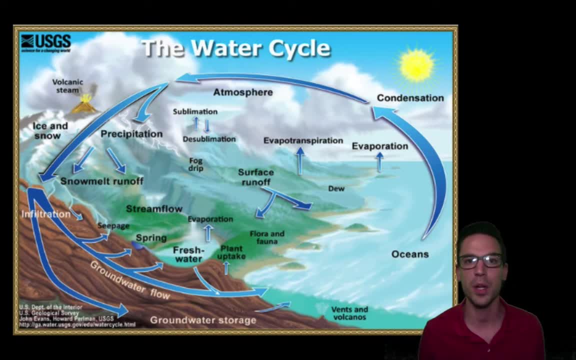 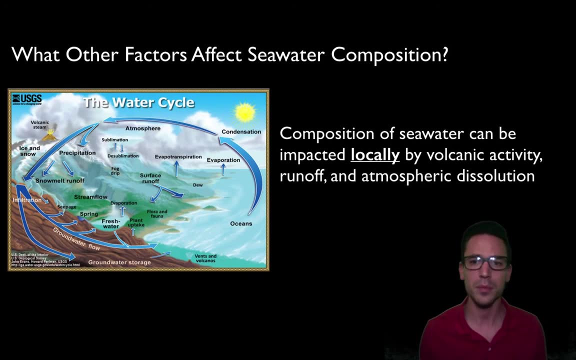 lakes and streams running off back into the ocean, And with that it's going to bring other various substances with it. So what other factors can affect seawater composition? Three major ones that we're going to take a look at are going to be volcanic activity, runoff and atmospheric. 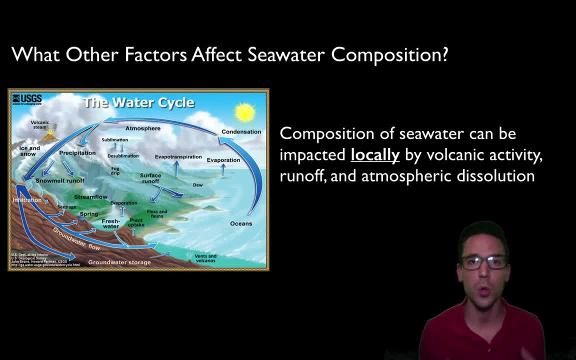 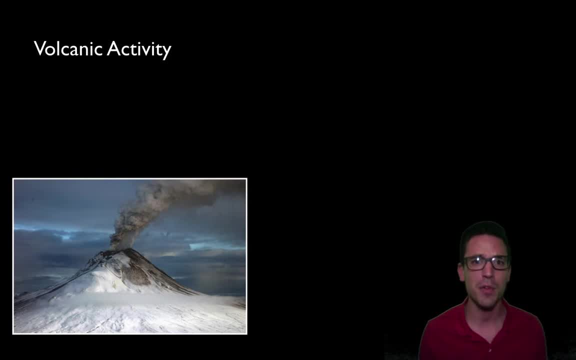 dissolution, And these things can affect the composition of seawater locally, In other words, in that area, wherever these things are occurring. So if we're to start with volcanic activity, anytime a volcano erupts, it's going to release gases out into the atmosphere. What's going to? 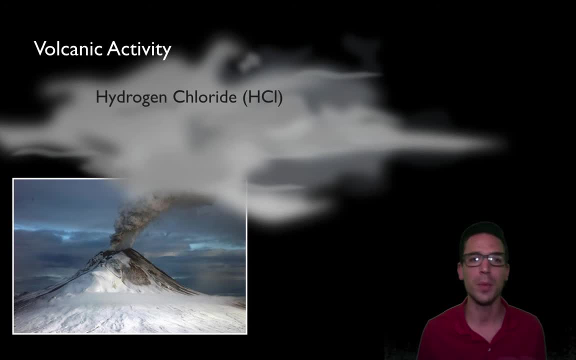 be inside those gases, or what sort of gases are we talking about? We're going to be looking at carbon dioxide, sulfur dioxide, hydrogen sulfide. All these gases are going to get released into the atmosphere. Now, what does this have to do with the oceans? Well, as these gases make their way, 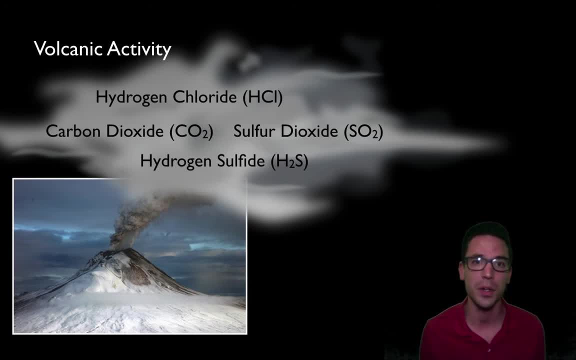 into the atmosphere. they're going to get dissolved in some of the water that's in the atmosphere as condensation and eventually they're going to precipitate. That means that they're going to make their way down into either the ground or into the oceans, but either way that's going to change. 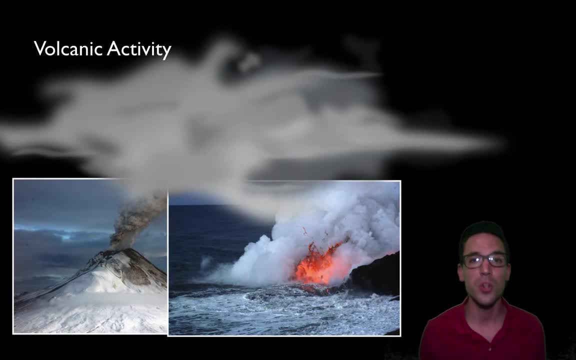 the chemical composition of water. The same thing even happens with underwater volcanoes. They're going to release the same sorts of gases and those things will get added into the oceans locally, wherever that volcano is located, One gas in particular that these volcanoes release. 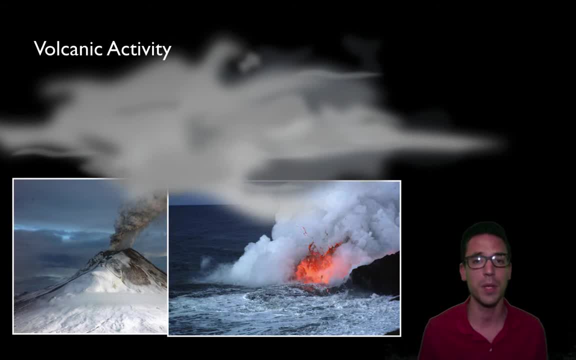 is chlorine gas. Now, if you get these, the chlorine being released, that's ultimately what's going to be a major source of those chloride ions we were talking about before. Remember that chloride ions make up the bulk of the salts. A lot of that chloride ions come from erupting volcanoes. 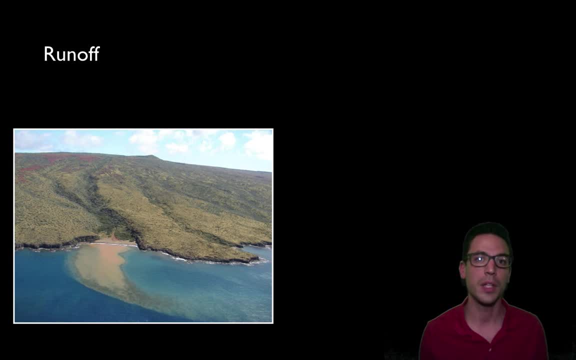 either underwater or above. Runoff will be another way that we can change the chemical composition of water. So all that runoff is is when water drains from land into the ocean. Now, this is a great thing, As water falls on land, as it runs off through groundwater along the surface. 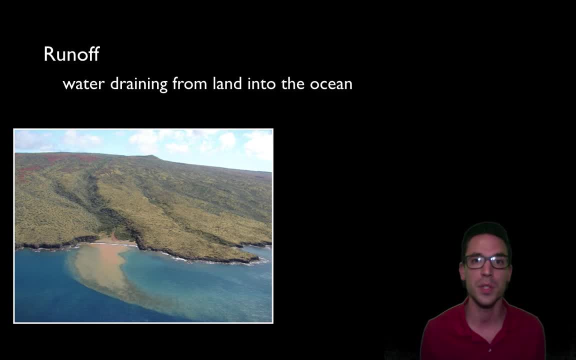 it's going to bring different nutrients with it: minerals, things that the organisms need to survive. That might increase productivity of, let's say, the phytoplankton, which will add more food and biomass for the rest of the food web. But another thing that runoff can bring with it and change the 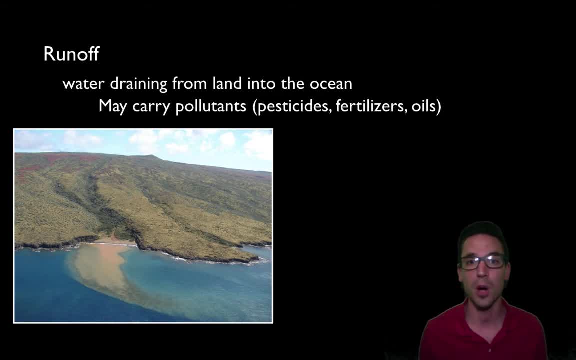 composition are going to be pollutants. So if that water runs through a nearby farm, it might bring pesticides and fertilizers with it. If that water comes from an urban area where there's a lot of cars and machinery and industry, that might bring oils with it. That might be a great way to get. 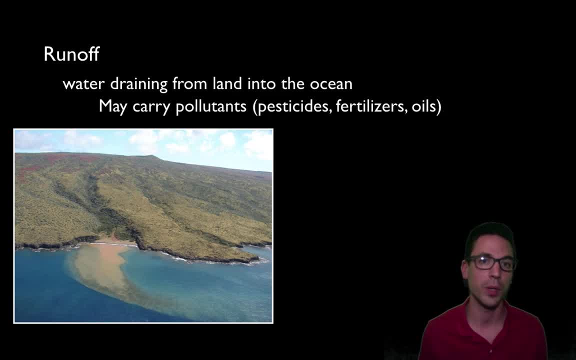 water to the ocean, And if you're in the ocean, you might want to get a little bit of water from the ocean, So that can have a negative impact on the local marine environment. Even if the pollutants are at a very low level, it's still a danger to the marine ecosystem. That is because of something. 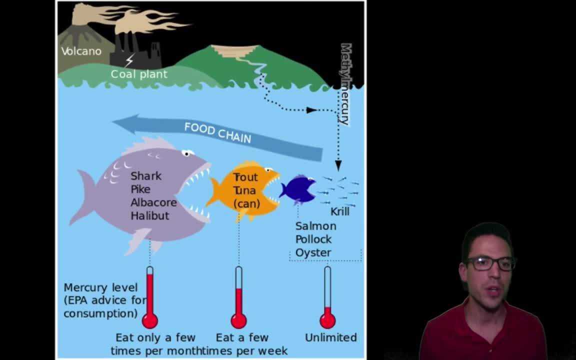 known as biomagnification. So we're going to look at this illustration here. Let's say this nearby coal plant is going to pollute or release these gases and in those gases are going to be something like mercury. Mercury is very toxic. Well as that, mercury makes its way into the marine ecosystem. 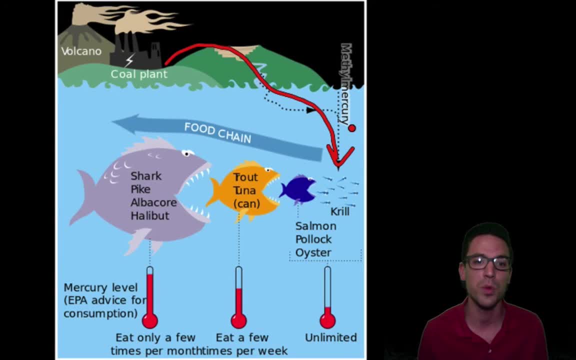 it might be at a very low concentration but it can build up as it moves through the food chain. So if just a little bit gets into the marine ecosystem, it might be at a very low concentration but it can build up as it moves through the food chain. So if just a little bit gets picked up by our 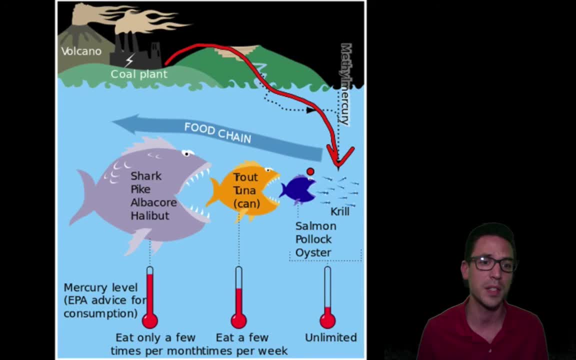 krill here. that krill might be eaten by a consumer. let's say a salmon. Well, that salmon is not going to eat just one krill. Let's say it eats a thousand krill, So therefore it's going to get a thousand. 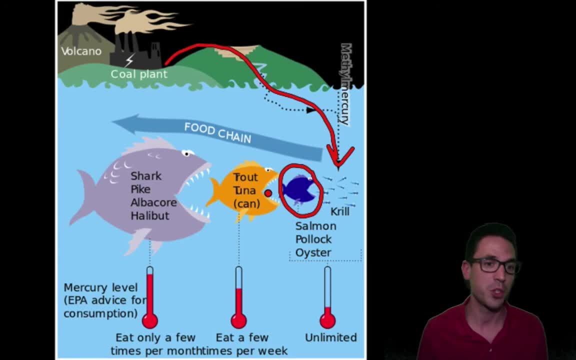 times more of that mercury inside its body. Then if a trout comes by and let's say, eats 10 salmon that have that now it's going to get a buildup of even more. And then when that trout gets eaten by a bigger, let's say a halibut here, a top consumer, it's going to get, let's say, eat 10 of those. 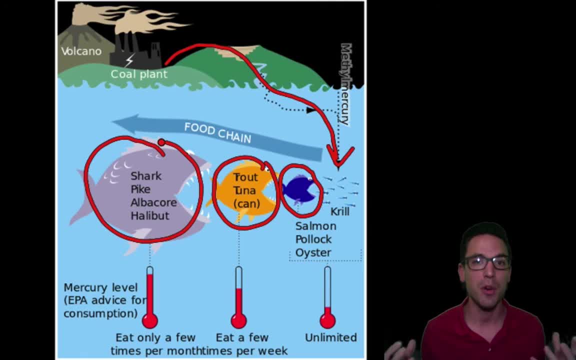 trout, it's going to get even more. So each step in a food chain the amount of mercury or any pollutants is going to build up even more. And then when that trout gets eaten by a bigger, let's say a halibut, it's going to get a buildup and we call that biomagnification. To magnify means to. 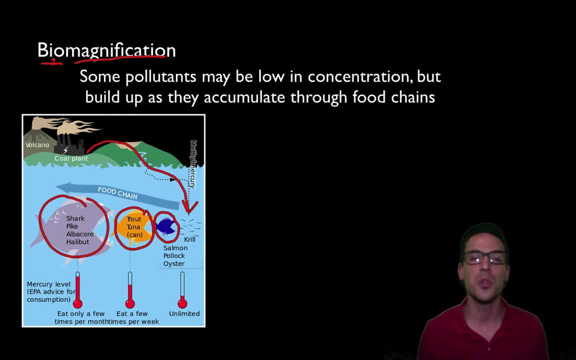 make bigger, and bio means we're talking about living things. So some pollutants may be low in concentration to begin with, but as it moves up through that food chain, it's going to build up and it's going to accumulate. One case that we saw this happen in history is the Minamata Bay. 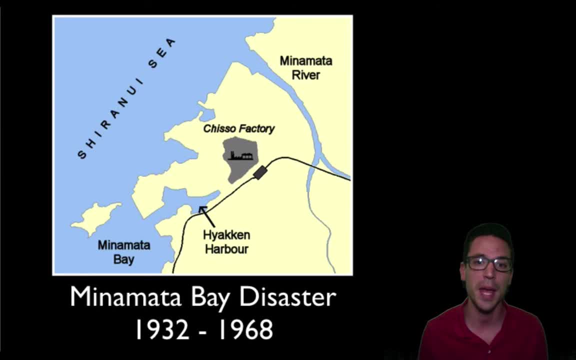 disaster. So Minamata Bay is a bay right off the coast of Japan And there was a factory, the Chiso factory, which is manufacturing fertilizers. What they were doing was: we're releasing mercury- low amounts of mercury- into the nearby Minamata Bay, which then eventually made its way into the food chain, And around 1932,. 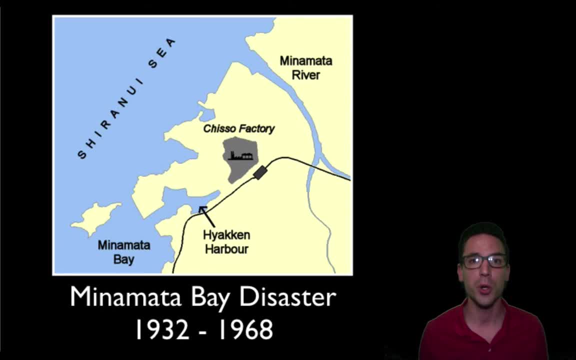 1968, people began to show symptoms of mercury poisoning, So having neurological disorders, paralysis and, in some cases, death. The cause of that was due to biomagnification through the food web, And eventually these people were eating shellfish and getting mercury poisoning from it. 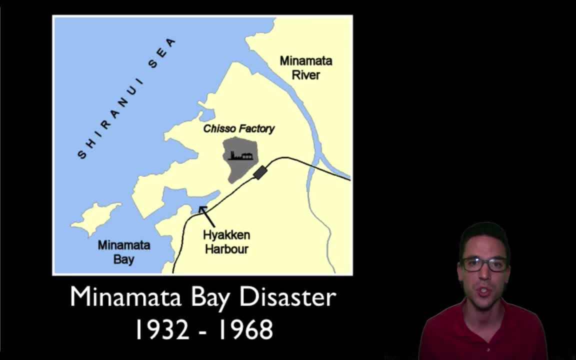 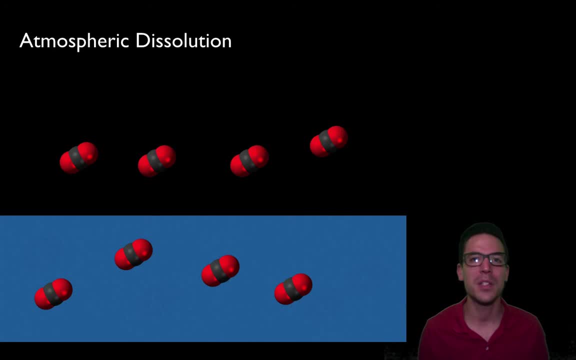 marine environment. Now, the final factor that we'll talk about that can impact seawater composition is gonna be atmospheric dissolution, or in other words, gases dissolving into the oceans from the atmosphere. Now, typically, gases in the atmosphere are gonna be at equilibrium with 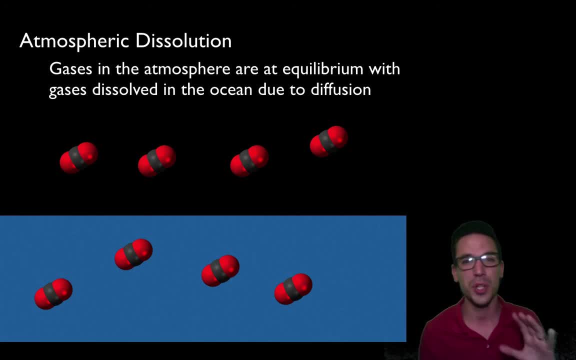 gases dissolved in the ocean just due to diffusion. In other words, there's usually gonna be about equal amounts in both, And that's because, as some gases move in and dissolve, some gases will move out. So here are some carbon dioxide atoms Every time one moves in. 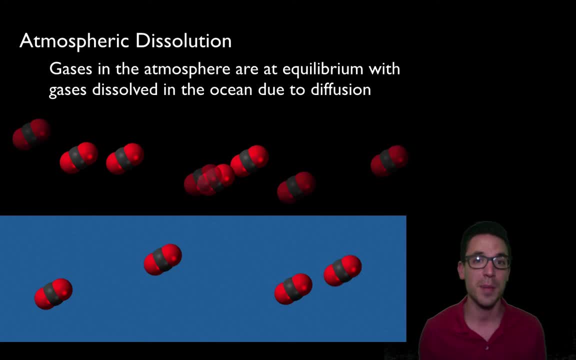 one might pop out, So they're always gonna have about equal. If I increase the amount of carbon in the atmosphere, that means more going to move in than out, so then eventually they'll balance themselves out. that'll increase the amount of gases inside the ocean. now what sort of things can impact this where we don't get equilibrium? well, 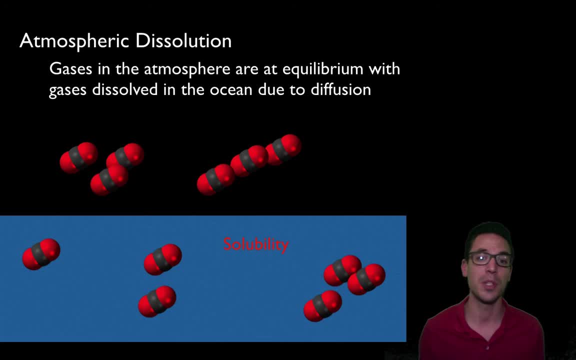 one thing is the solubility of the gas. some gases are more able to dissolve in the oceans than others. so if it's not able to dissolve well, it's not going to have a high concentration inside the oceans. if it's easily dissolves in water. 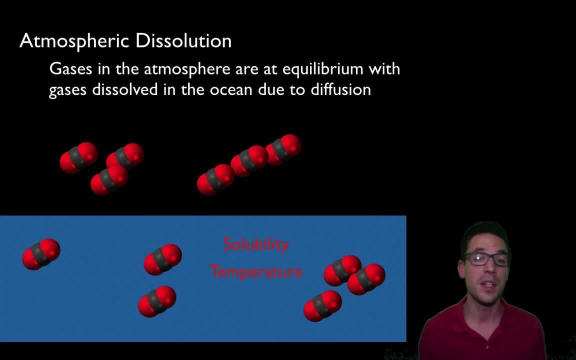 we'd expect more of it inside that water as it dissolves in. the temperature of the water can also impact this, so typically colder temperature water can hold more gases than warmer temperature. so we're usually going to find more, let's say, oxygen and carbon dioxide in the polar areas than in the tropical. 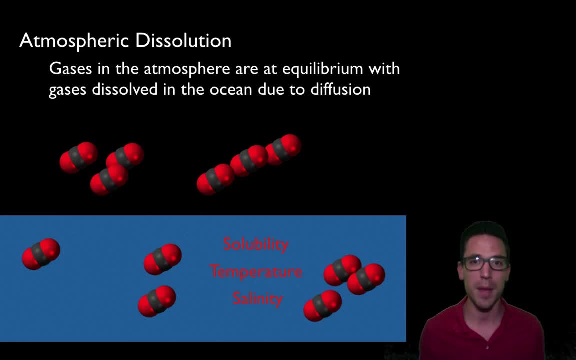 areas where the water is warmer. and finally, salinity. the amount of salts will impact it. the more salt or the more salinity, or the higher the salinity, the less gases it can hold. less salinity or the lower the salinity, the more gases it can hold. now, what gases are most dissolved in oceans that you need to be? 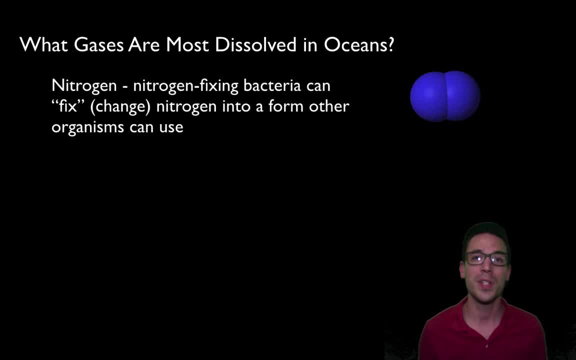 most concerned with. there are three big ones that you should know. the first one is nitrogen gas. that nitrogen, as it makes its way into the oceans or dissolves in, they're going to be bacteria that can fix it. or in other words, take that nitrogen and then change it into a form that other 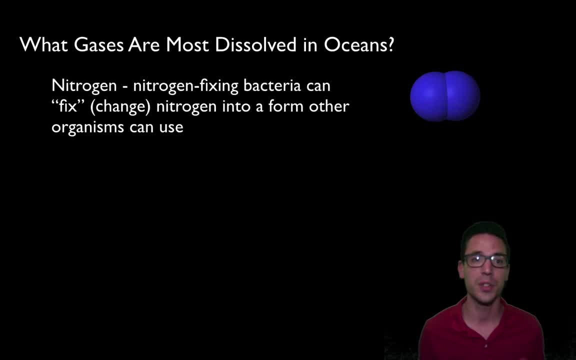 organisms can use. why do we need nitrogen? well, all organisms use nitrogen for their DNA, they use it for proteins, so without nitrogen, organisms can't live. another important gas is oxygen. as you're aware, without oxygen you can't live. we need it for respiration so as that oxygen dissolves into the oceans. 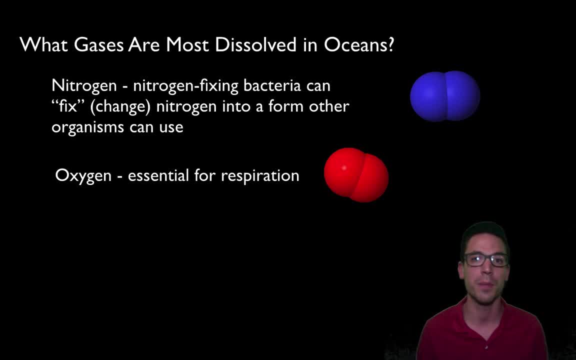 organisms can then use that oxygen to do cellular respiration and then, finally, the oxygen is then used to make the nitrogen gas, especially in the process of photosynthesis. we're going to use that and that's going to kick off the productivity for organic compounds that other organisms can use. so at this point,